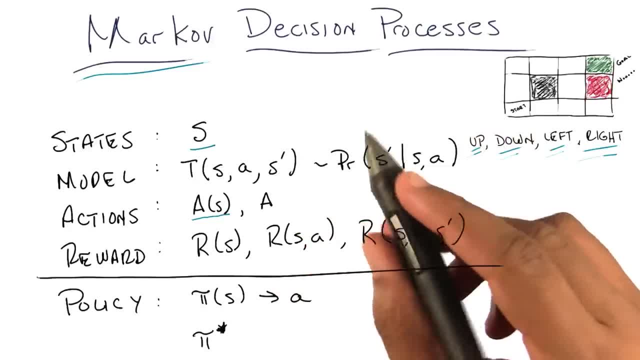 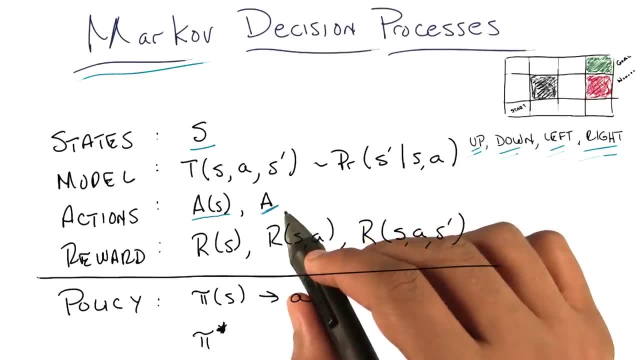 being a function of state, Because there are some states you can do some things and some states you can't do those things. But most of the time people just treat it as a set of actions And the actions that aren't allowable in a 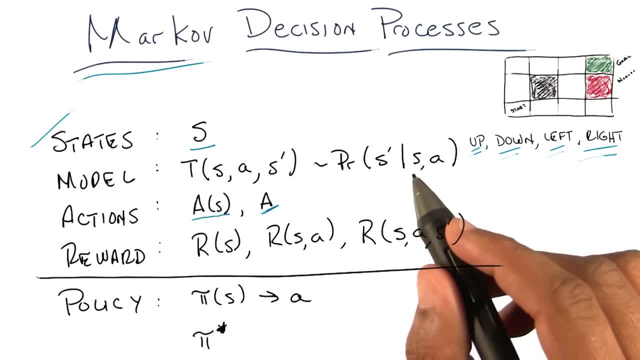 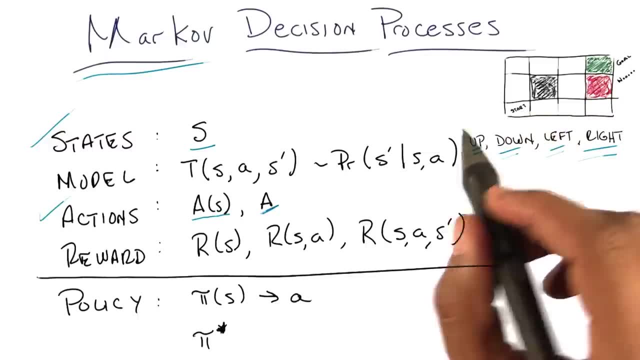 particular state are the actions that are allowed to be done. States simply have no effect. All right, so we understand states. They're the things that describe the world. We understand actions. Those are the things that you can do, the commands you can execute when you're in particular states. 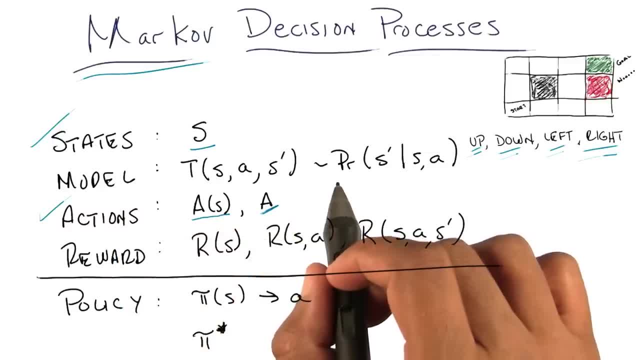 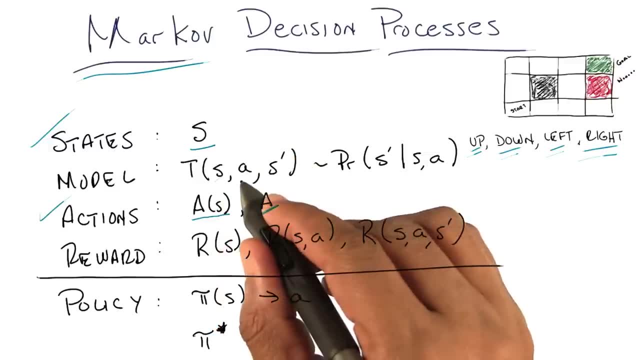 And what a model describes. what the transition model describes is, in some sense, the rules of the game that you're playing. It's the physics of the world. So it's a function of three of three variables: a state, an action and 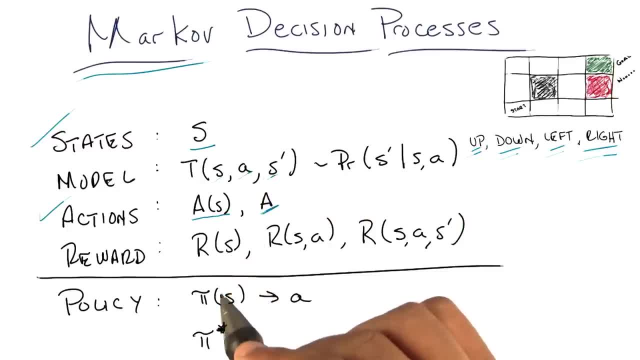 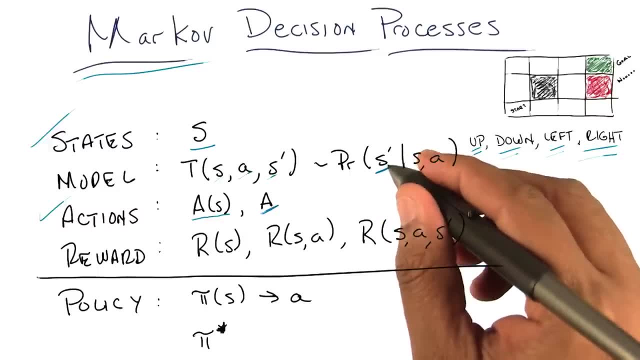 another state, which, by the way, could actually be the same state, And what this function produces is the probability That you will end up transitioning to state S prime. given that you were in state S and you took action, A Got it. 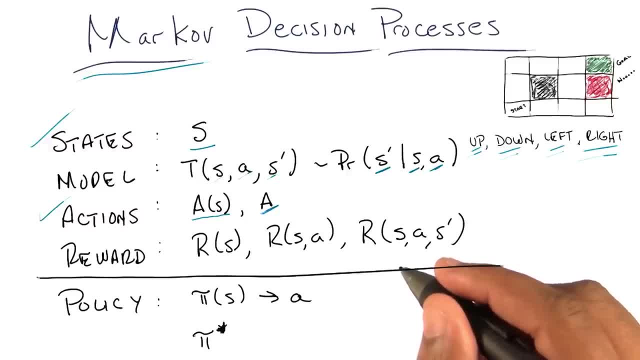 I think so. So the S prime is where you end up and the SA is what you're given. So it's so. you plug these three in, Oh I see, and you get a probability out, Mm-hm. 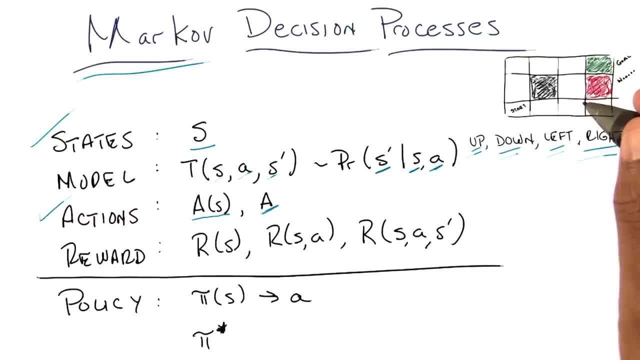 But the probabilities have to add up to one. if you, if you sum it up over all the S primes, Right, That's exactly right. So, for example, if you think about the deterministic case where there was no noise, then this is a very simple model. If I'm in the 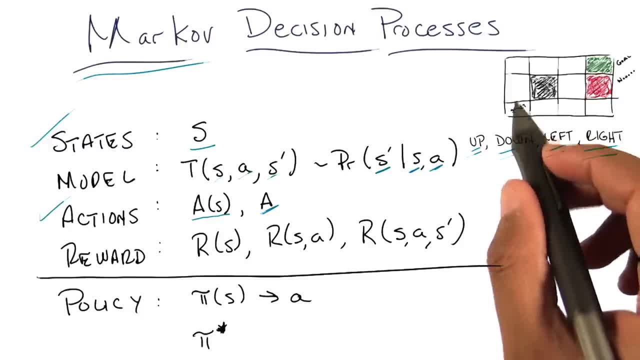 state, the start state, and I take the action up, then what's the probability I end up in the state immediately above it. Was that a 0.8?? No, in the in the when we first started in the deterministic world. 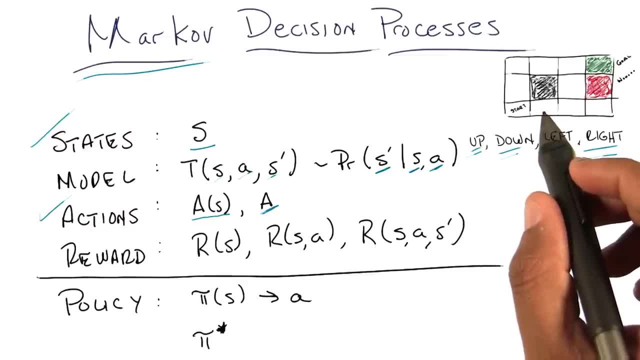 Oh, that was probability one, Right. and what would be the probability? you ended up in the state to the right Probability: zero, Right. In fact, the probability that you end up in any of the other states is zero in the deterministic world. Now, what about the case when? 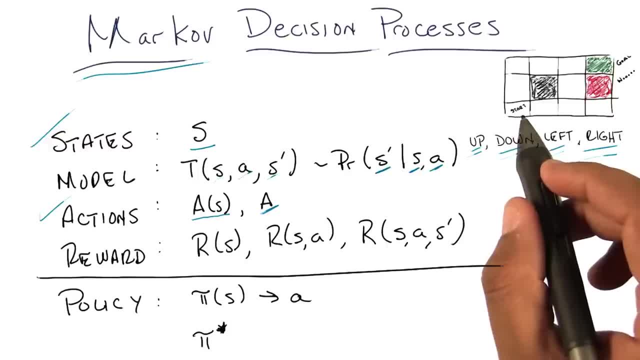 We were in the non-deterministic world where an action would actually execute faithfully only 80% of the time. If I'm in the start state and I go up, what's the probability that I end up in the state above? That was 0.8.. 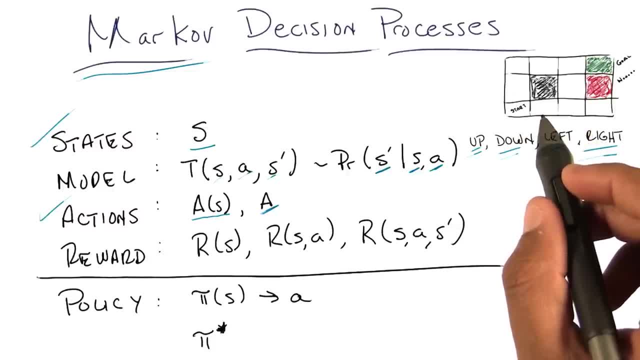 Right. What's the probability I end up in the state to the right. That was 0.1.. And what's the probability I end up where I started? That was also 0.1.. Right and zero everywhere else, And that's just sort of the way that it works. 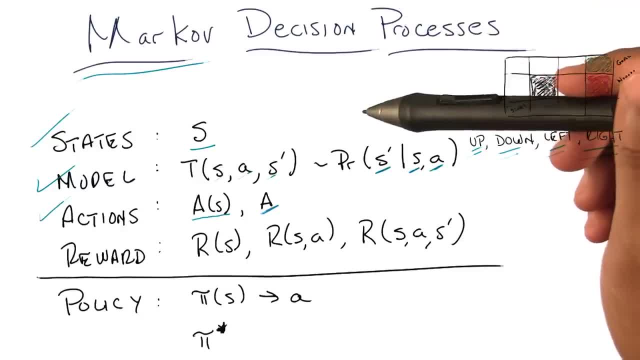 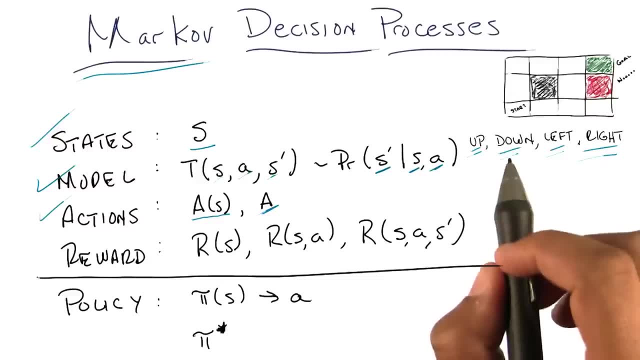 So the model really is an important thing, And the reason it's important is it really does describe the rules of the game. It tells you what you, what will happen if you do something in a particular place. It captures everything that you know about the transition of the world, what you know about the rules.